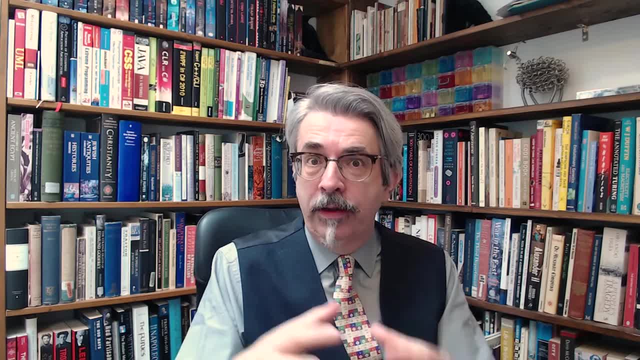 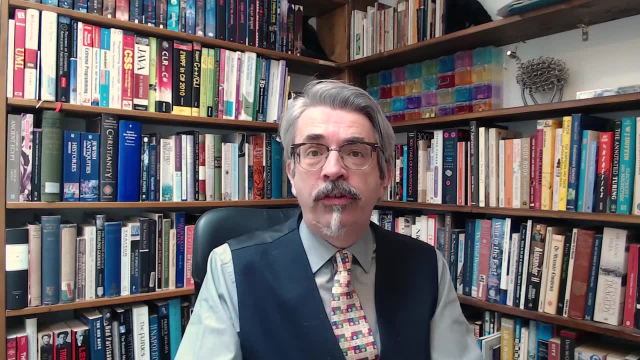 although we can use this in collaboration with the Composite Pattern, and that's what I'm going to show you today. it is useful with all sorts of different data structures When you've got a situation where you have the potential for a lot of duplicated data. the key idea behind the 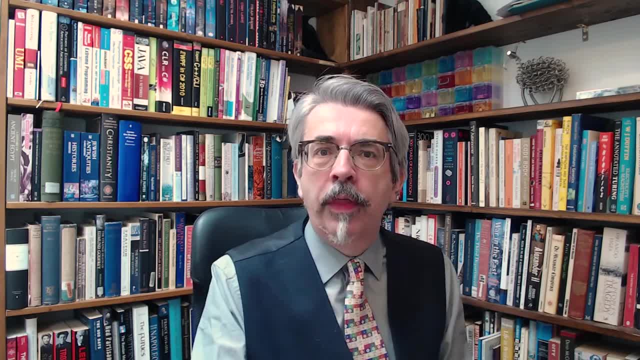 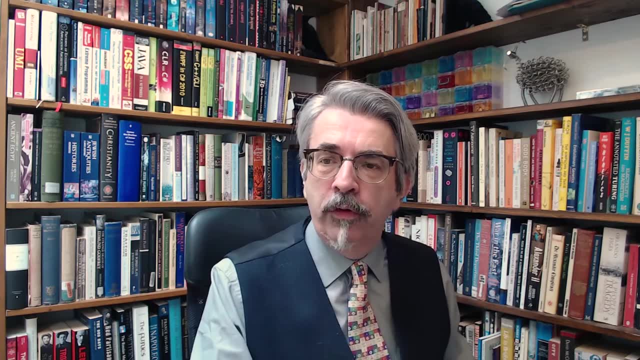 Flyway Pattern is to save memory. So let's have a look at what we've got there. And, going back to the Composite Pattern that I showed you, I've made a few changes just to get things on a better footing for this. So if we look at our program, the main change that I've made here is rather: 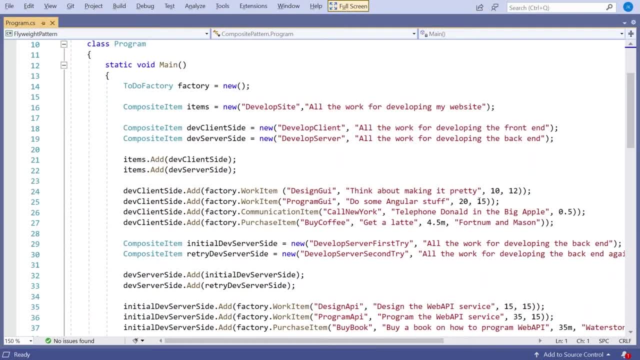 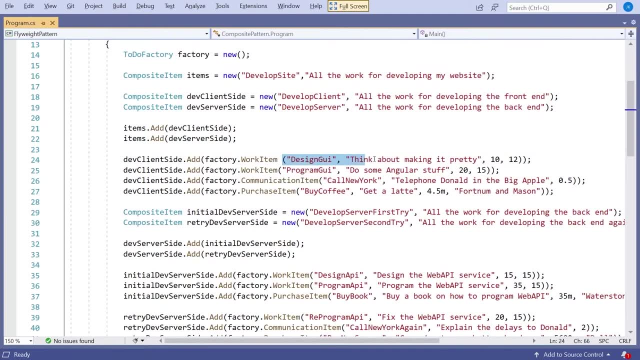 than having those predefined work items and communication items and that sort of thing, I've actually created these directly in Mac. So there we've got a work item for design the GUI. There we've got a purchase item for buy coffee and that sort of thing And also, rather than calling new, directly there, 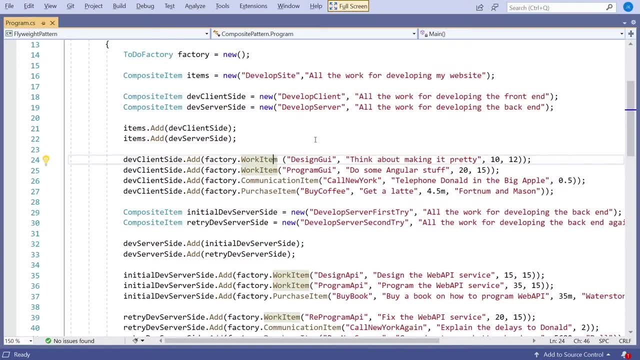 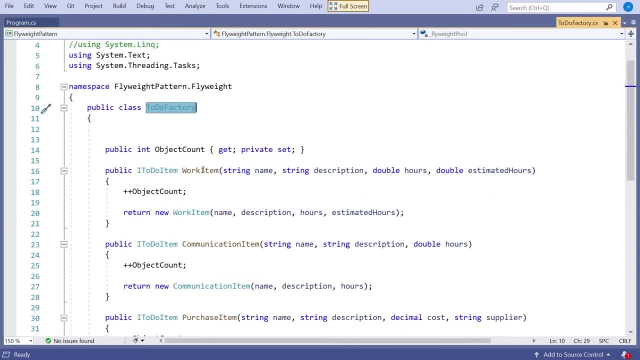 I'm starting to create these through a factory And that's going to be necessary when we see how this Flyway Pattern works. But the thing that we have with our factory it's pretty simple. We just ask for a work item or a communication item or a purchase item and pass in the data. 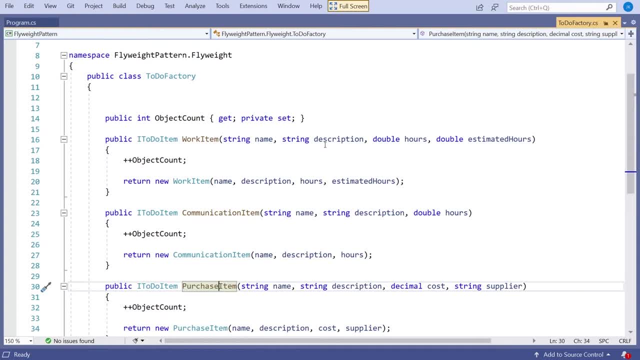 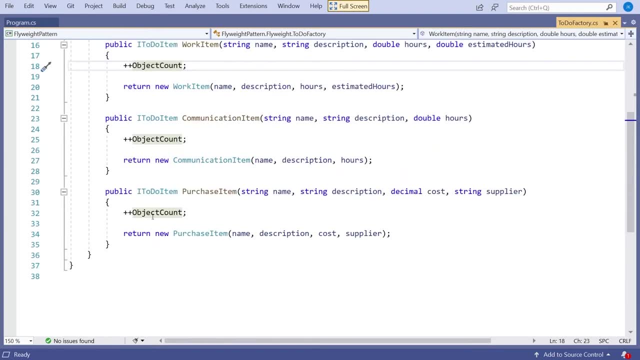 But one thing I've put in here already, which is really just to demonstrate the benefits of this pattern. You wouldn't have it in real code, But I'm just keeping an object count of how many total objects we've created, And then at the end of all this I just print that out. 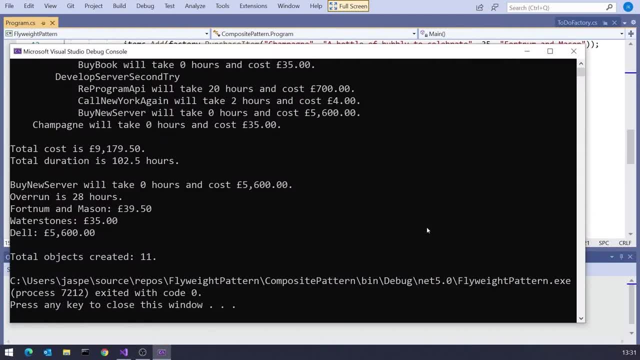 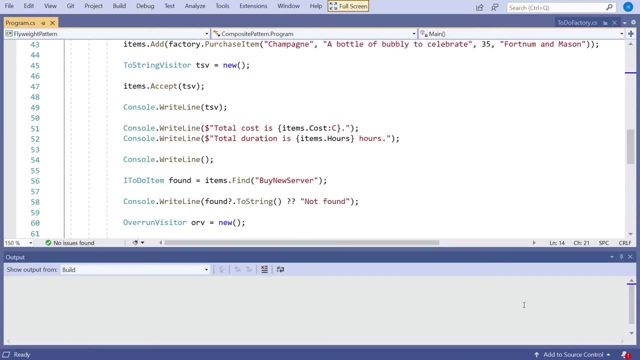 So if we run this, we can see it's doing all exactly the same thing it did before. But then we've got this: total objects created of 11.. So that was all of the different items. But the thing is, if we take a look at this, we might decide that just having coffee the once. 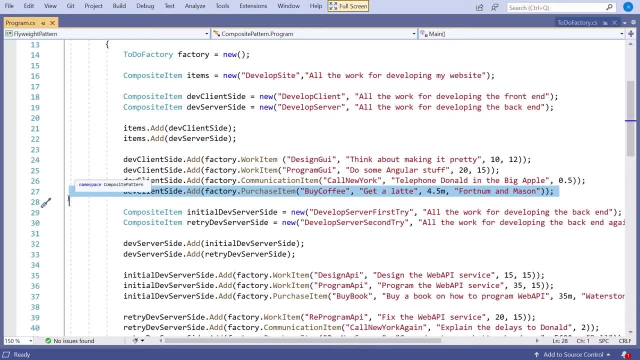 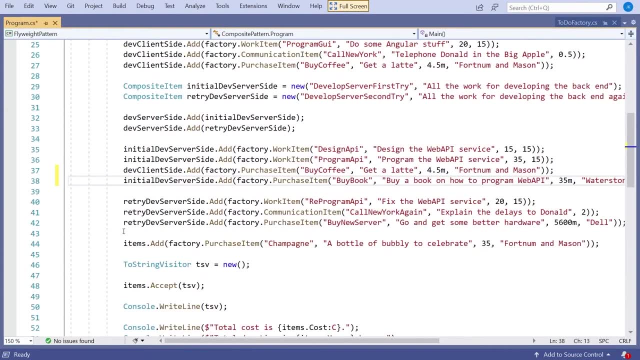 is not a good idea. It's not really how things are going to be. We're going to be buying coffee several times, So if I copy that, let's also have a cup of coffee before we buy our book, And let's have a cup of coffee before we call New York. 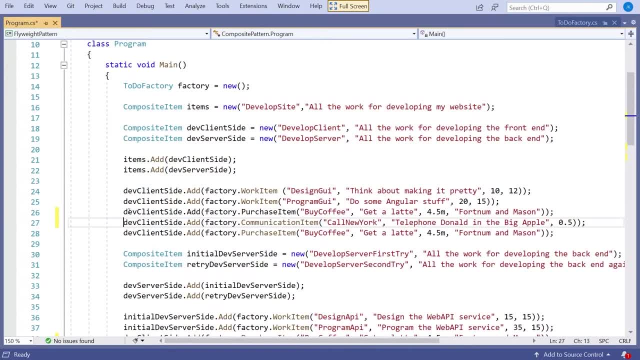 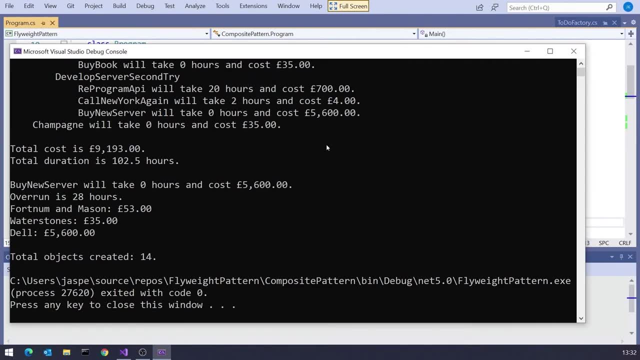 And in fact let's have another cup of coffee before we call New York there as well. So I've created four purchase items of Buy a Cup of Coffee And if we take a look at that then we can see we've now got 14 items created. 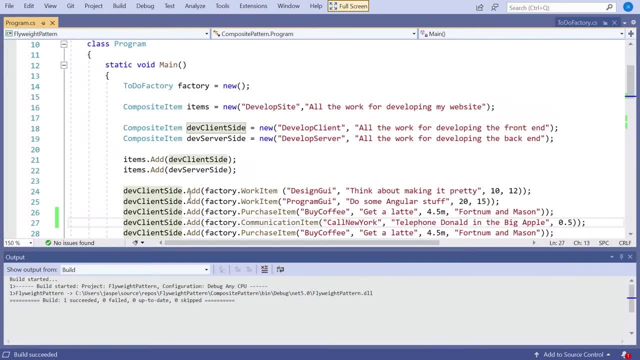 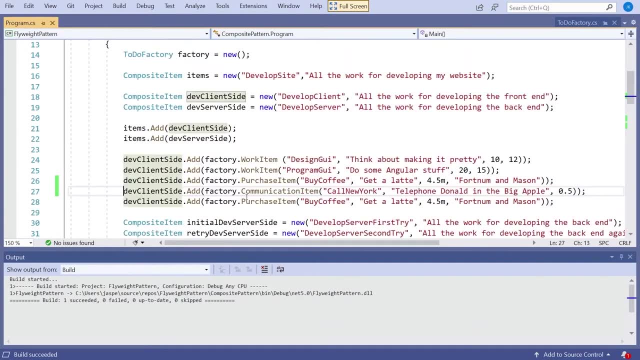 And we've got a slightly different structure with all that coffee. But the thing about that is you might think that is slightly wasteful, Because all of those coffee items are exactly the same. It's the same coffee, the same price, the same supplier. 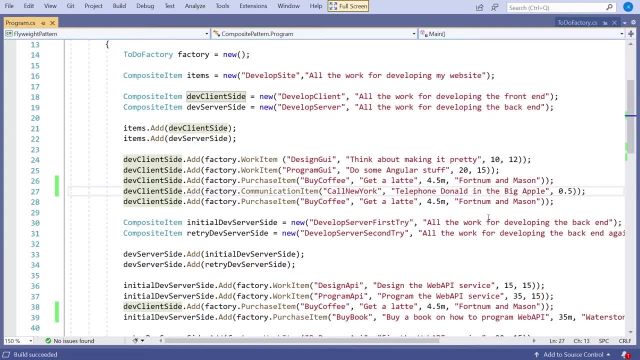 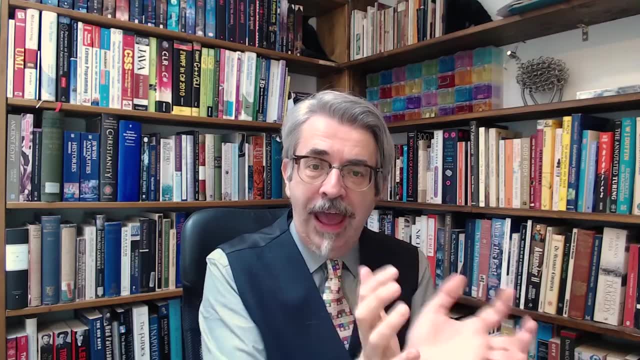 Might not be, of course, but in this case it happens to be, And so why do we need to duplicate? that- And that's the key idea of the Flyweight Pattern- is, when you've got a structure like Composite and you have shared data across nodes, you can save memory, if you actually 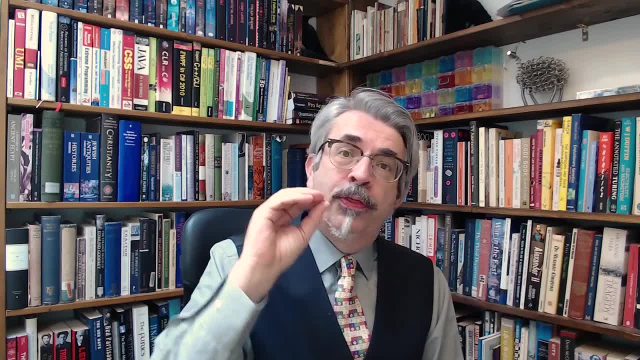 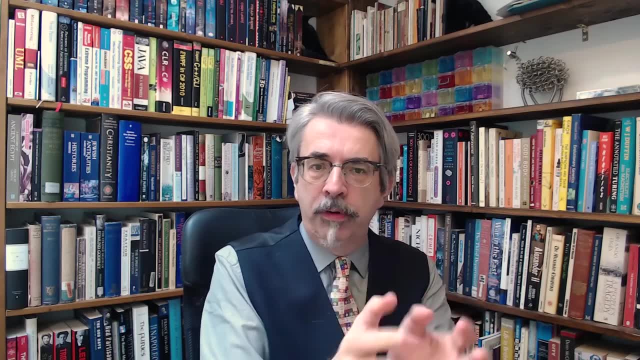 have shared nodes rather than just shared data. The thing to bear in mind about it is that's only going to work if these things are immutable. If it were possible to change, say, the price of a coffee, then if that were being shared. 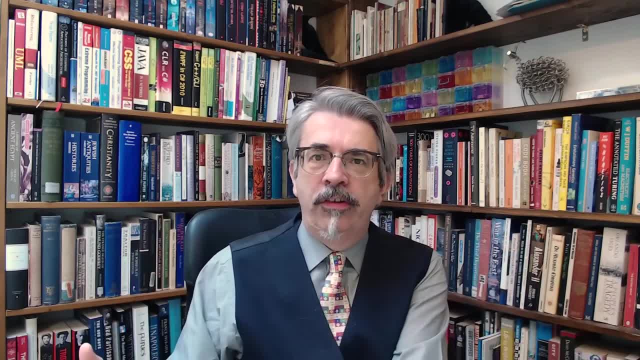 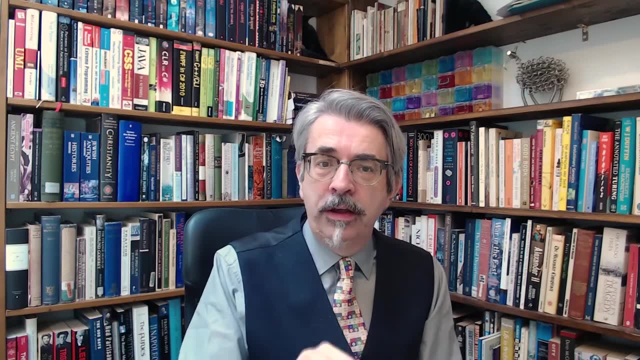 across the structure, then you change it in one place, it changes it in another place, and that shouldn't happen. They should remain separate objects. So that's why these items have to be immutable And, as we saw in an earlier video, in this case, if you have two coffee items, one of them has a smaller amount of energy, like one of the other will do. 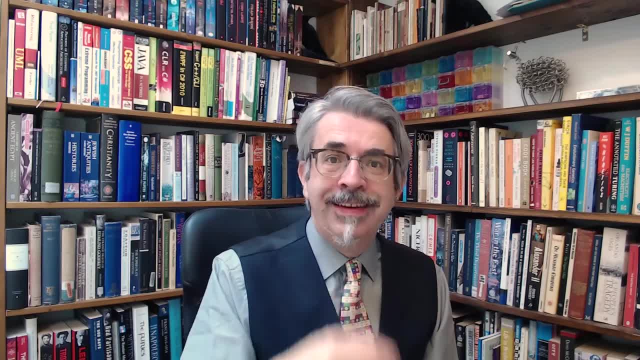 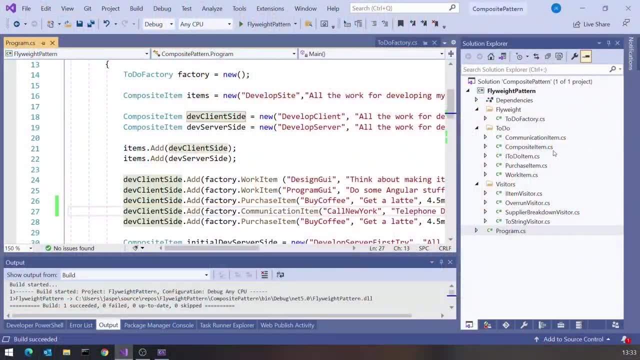 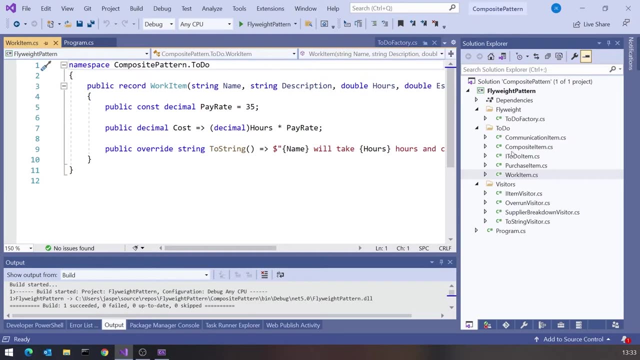 an earlier video in C-sharp 9, which I've got here. the neat way to create immutable objects is to have them as records. So that's actually another change I've made here, that if we look at each of our derived items, we have these as records. So there's our work item, there's our. 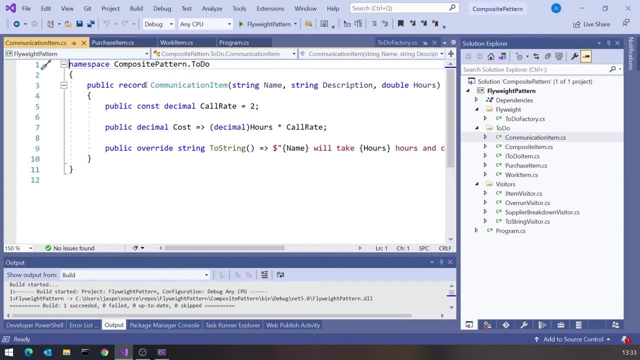 purchase item, there's our communication item, and nothing really different if you compare that to what we had before. except they're implemented as records, not as classes. My composite, however, still needs to be a class, because the composite isn't going to be immutable. That's how we structure. 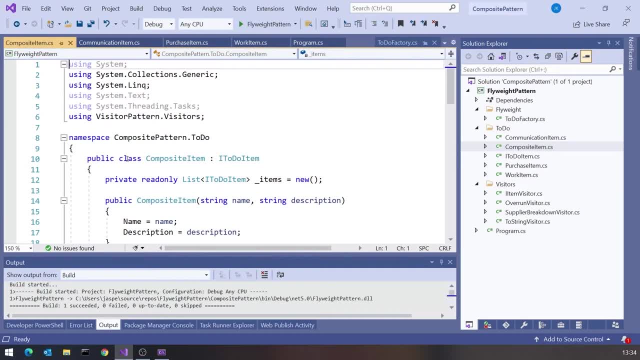 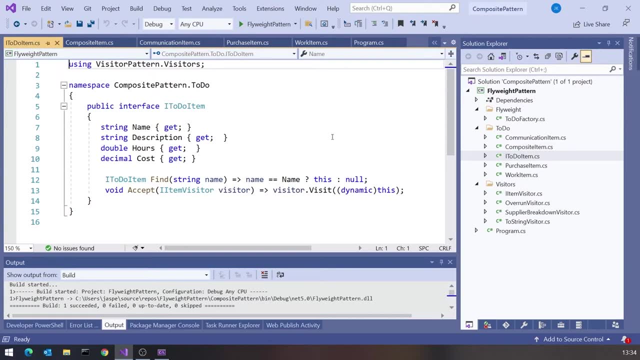 all these things. so the composite itself doesn't get really featured in this flyweight, And for that reason we've also had to change the root item, the to-do item itself, to an interface, because you're not allowed to derive a class from a record or a record from a class, so we've got to have an. 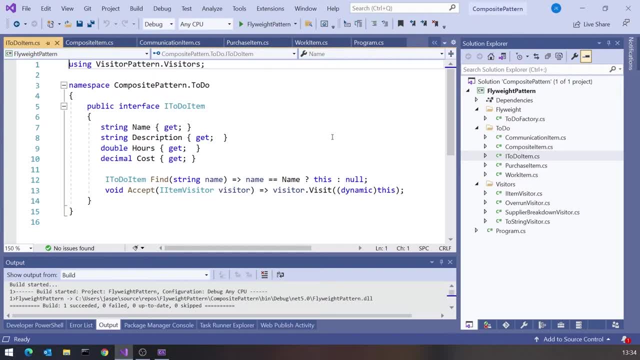 interface there so that the leaf item doesn't have to be a class. So we've got to have an interface there so that the leaf item can be records and the composite can be a class. So no real changes in behavior there as yet, it's just introducing these records. And the thing about records is they give us two features. 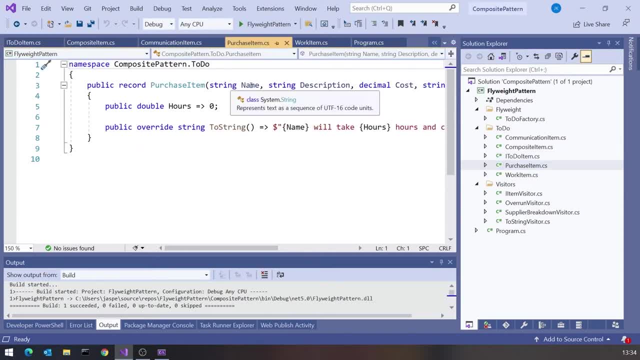 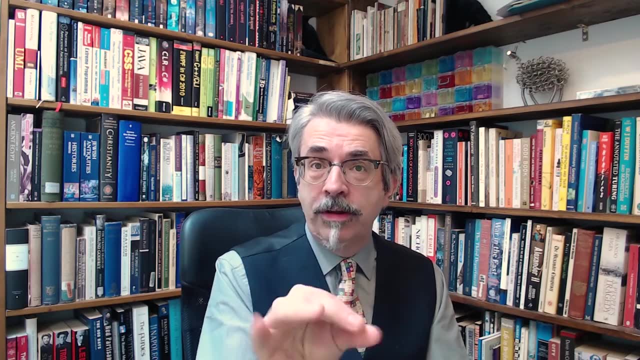 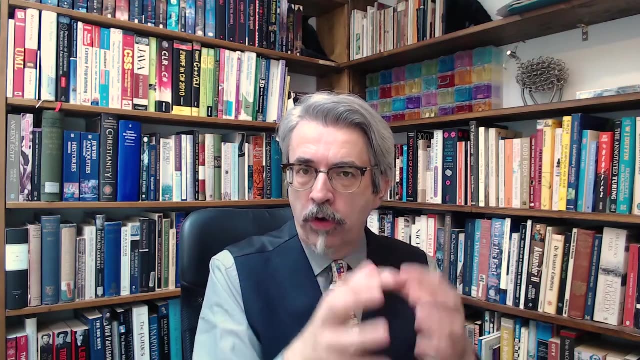 actually We get the fact that they are immutable, so once we've set up this purchase item we can't change it. but also it gives us an automatically overridden equals method so that we can compare these items on a value basis- not on a reference basis, but on a value basis. 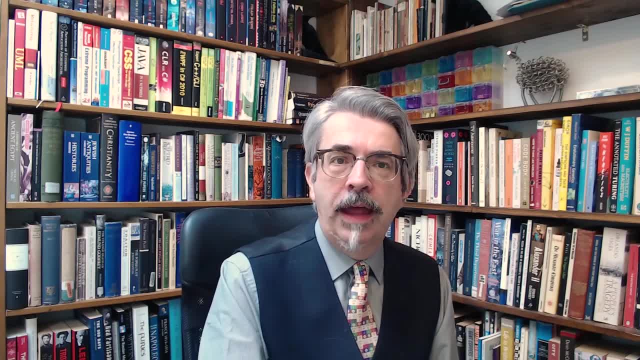 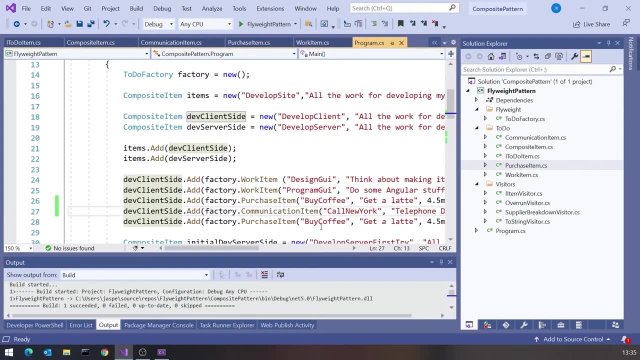 Which is again what we want to do here, because we're saying that those two coffees are duplicates because they have the same value, even though they're different things. So what do we do? Well, we go to our factory and we introduce in here what is known as a flyweight pool. 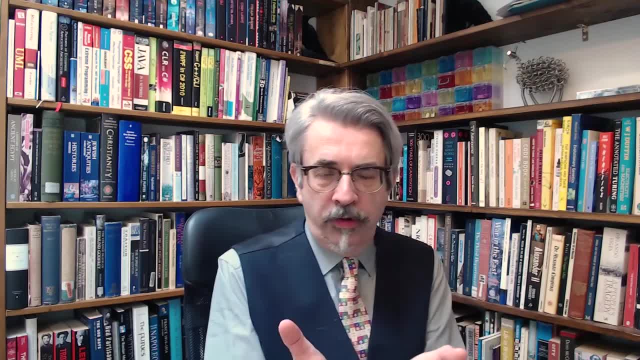 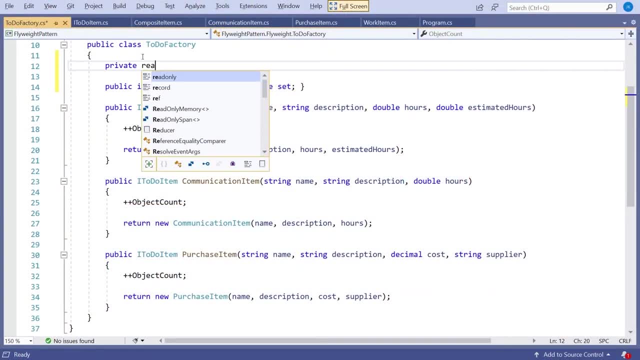 So this is where we're going to store all of the objects that have been created, so we can hand them out instead of duplicates. So we will have a private read-only, and I'm going to use a class called hashSet here, which is the ideal one for this purpose, which just allows us to store these. 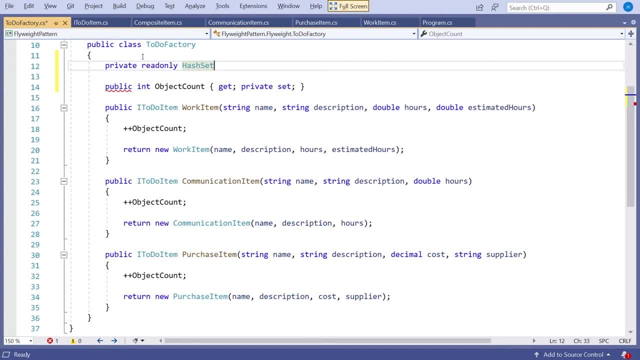 things and look them up on the basis of that value equals. And so this is going to be a hashSet of iToDoItems and we call this the flyweight pool and just create it. And then, for now, let's just start this with the purchase item, because that's the one we've got duplicates on. 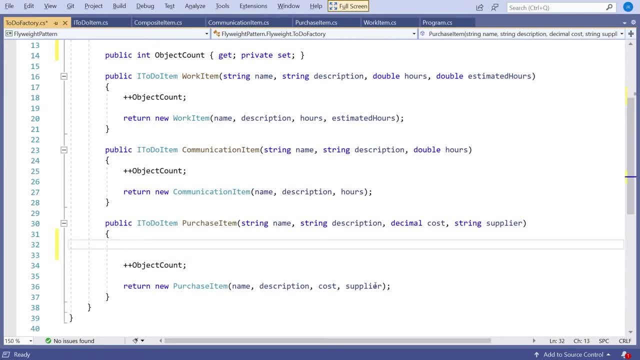 So what I'm going to do here is actually I'm still going to create my purchase item, So we'll call this newItem and then just pop into there that actual creation. But this is only going to be temporary if we've already got one of these. So remember, we're trying to save memory. 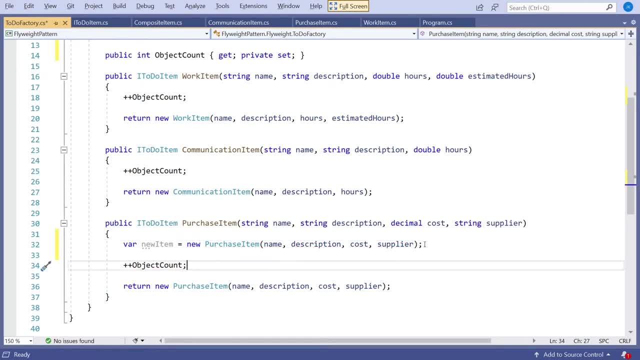 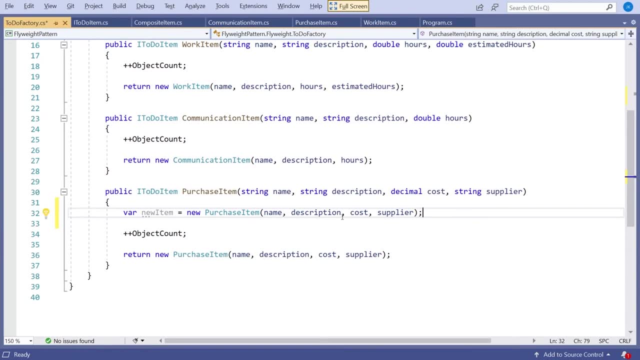 so it's okay to have that for a short period of time, And then what we've got to do is see if there is already a new item that we want to create. So we're going to click on that and we're going to create a matching item in our hashSet. So what we can do for that is we say if, and then 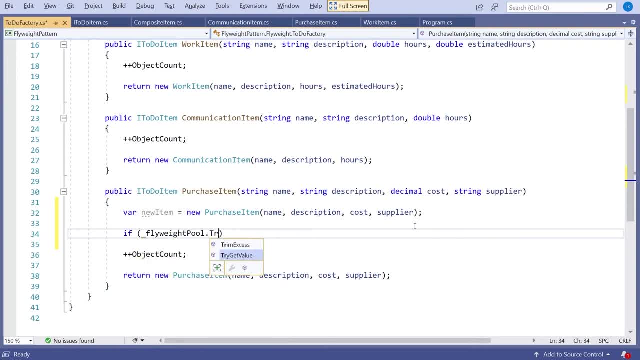 underscore flyweight pool and that has a method called tryGetValue. So what that does is allows us to look up a value which matches newItem. It's going to match it using this automatically generated value-based equals method that we get because it's a record. 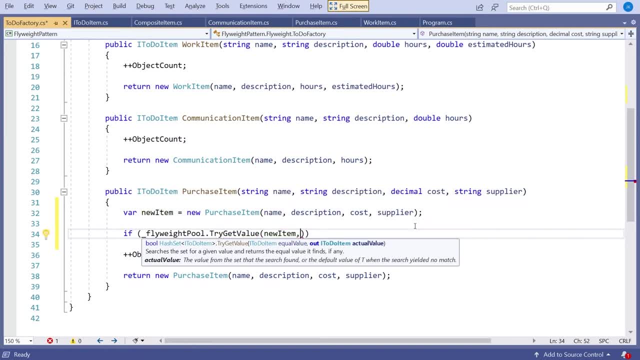 And then we're going to get out either the item that matches inside the hashSet or if there's nothing there, it'll just return false and give us back null. So we can say out var and then let's have foundItem And if it does, find an item, 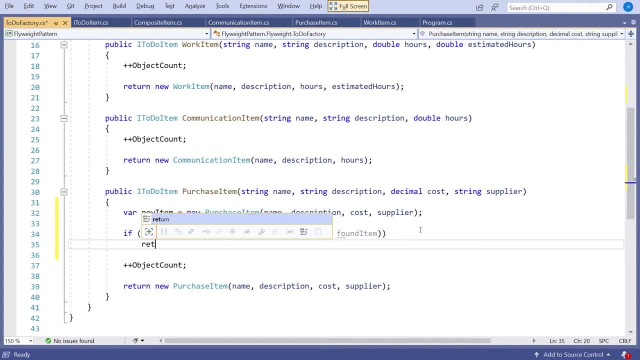 so if tryGetValue returns true, then we simply return that foundItem, In which case the newItem will now not have been stored anywhere, it'll be up for garbage collection, we don't have to worry about it, Whereas if we haven't found it, 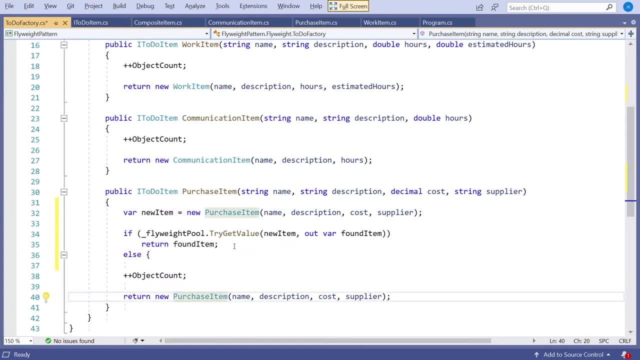 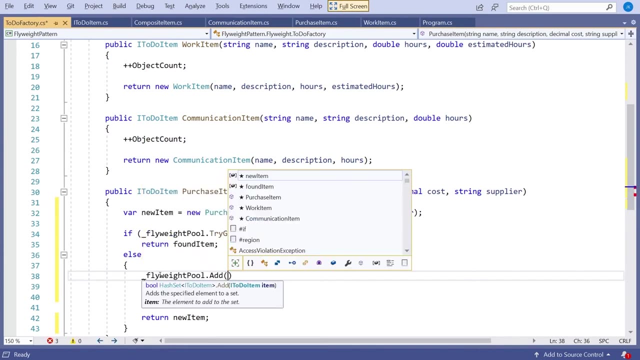 then that means we're going to need to return the newItem, We're going to obviously need to increment that objectCount because we've created a newItem that we're going to use now And also we've got to add it to the flyweight pool so that next time it will get looked up correctly. 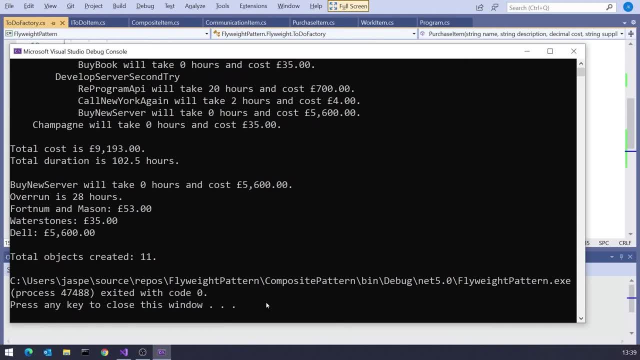 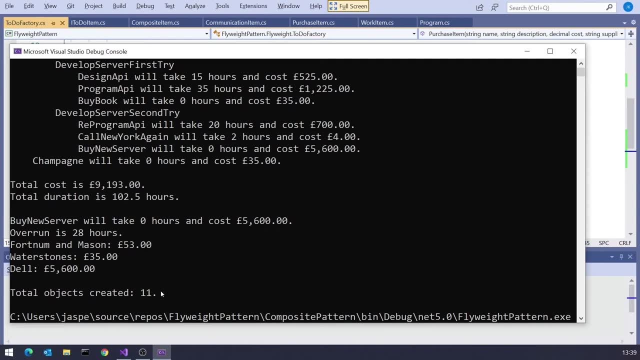 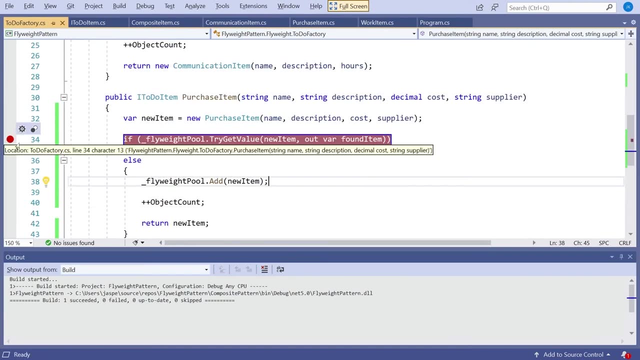 And now, if we do that, if we run that, we can see that, although it's behaving the same way, we've still got all those coffees. it's now back down to 11 rather than the 14, because it's only created the one. We can just take a quick look in the debugger. So in here. 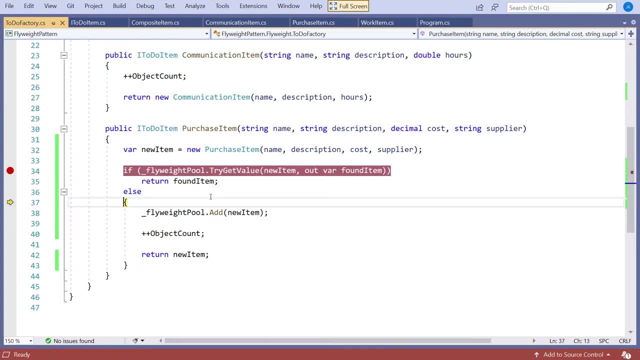 first time we come in, we create a newItem. it doesn't find it. so the newItem that we created, we add to the pool, increase the count and return it Next time around we create the item, but then we discover we've already got one in there. 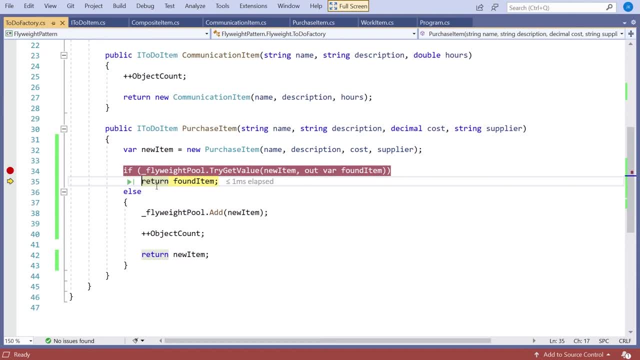 so we return the one that we found. The newItem will disappear when it gets garbage collected and that's going to be the same on all of the subsequent ones, presuming it's the same item. Obviously, when we purchase something else, like the server, that will not match up, But that's the 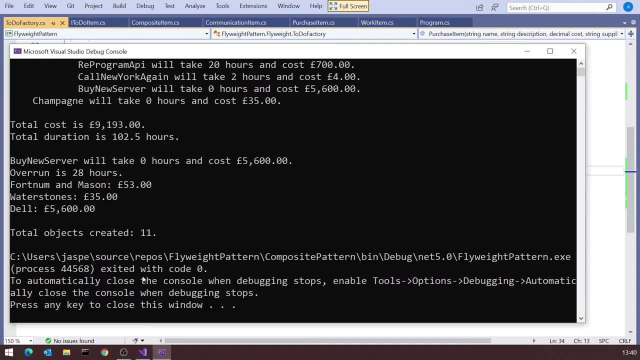 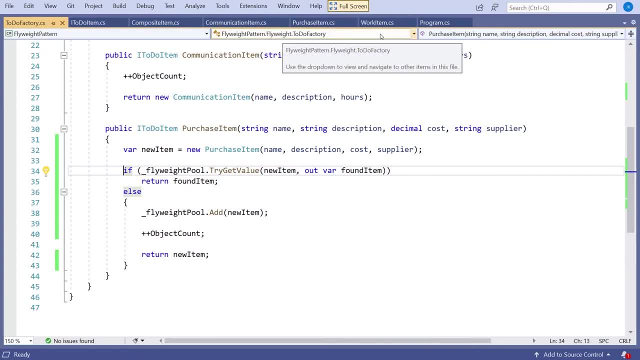 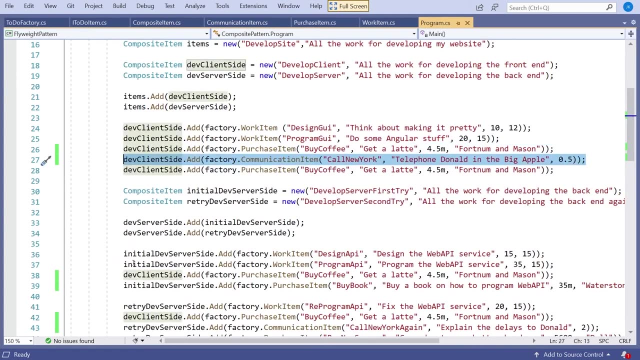 basics of how it works. So now we could just go through that and do the same in each one of the others. So let's put in some other duplicates, Just so we can see it working. So let's have a duplicate telephone call, So let's put that into. 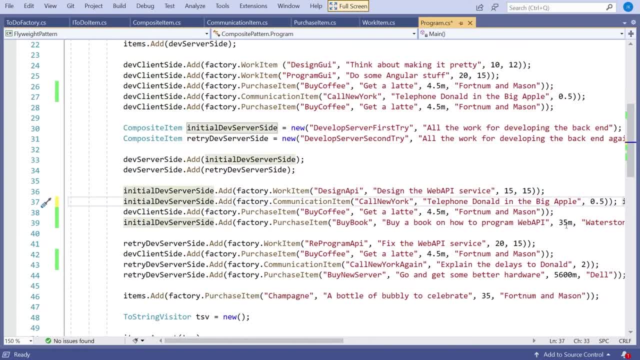 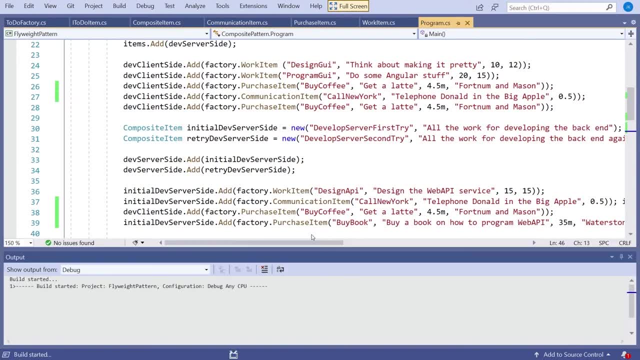 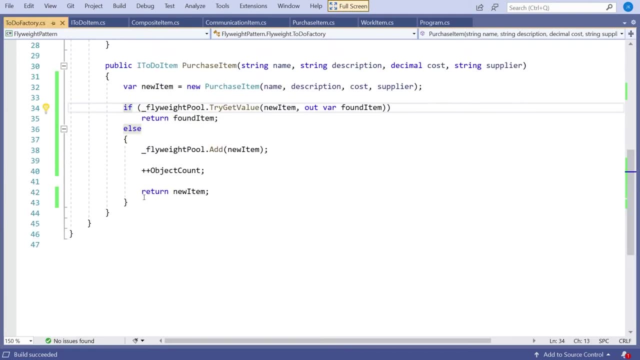 there And let's have a duplicate work item. Put that on the end there And once again, when we run that we'll see that we're getting too many objects- 13 of them now. So essentially it's just going to be cut and paste.